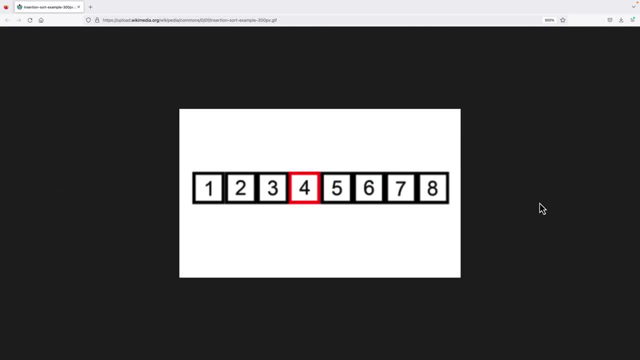 algorithm. We do this until we reach the end of the array and no more unsorted elements remain. Now, initially, in this example, six would be the sorted portion of the array. We would then look at the element five and insert it into its correct position in the left-hand sorted portion of the 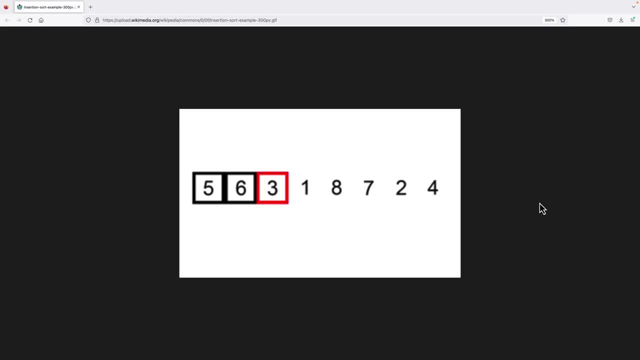 array. Then next we would look at three and insert it into its correct position in the left-hand sorted portion of the array. And then we look at one and insert it into its correct position, Sometimes like one, if the element is less than all the elements in the sorted portion of the. 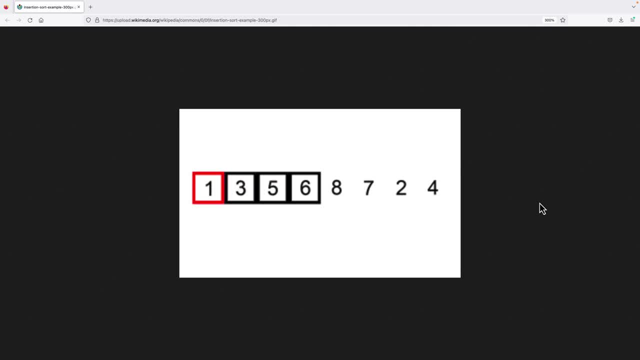 array. it will be inserted at the very front of the array. Sometimes an element like eight here doesn't need to move at all to go into its correct position. We call the element that we are currently looking at in the unsorted portion of the array the key, In order to insert the key into its correct 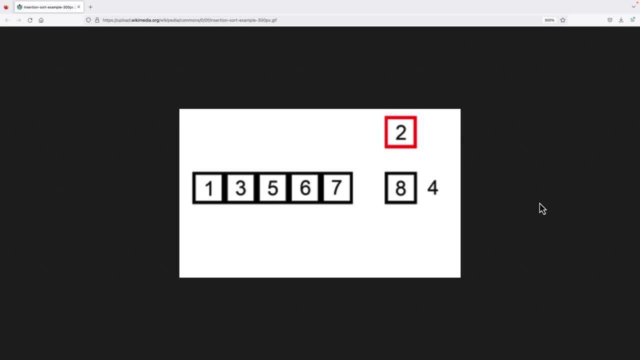 position in the sorted portion of the array. we continually shift over the elements in that left-hand sorted portion of the array by one index until we either reach the start of the array or we find an element in the sorted portion of the array that is less than or equal to the key, at which point. 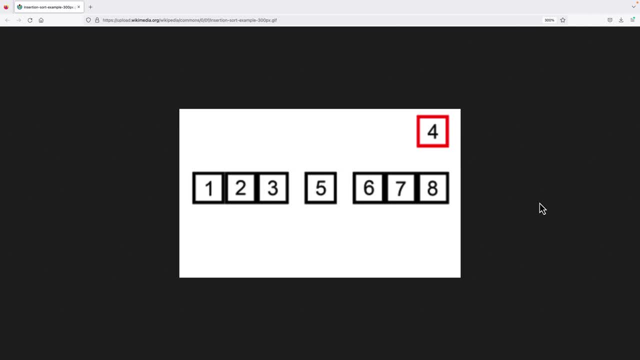 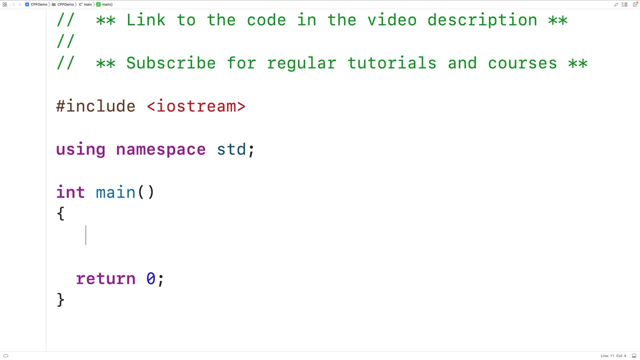 we found the right spot for that key to be inserted. So here, three is less than our key four, so we found the spot where four belongs. Let's actually implement this algorithm in C++ now. So the first thing we'll do is declare an int array called a. We'll initialize this array with: 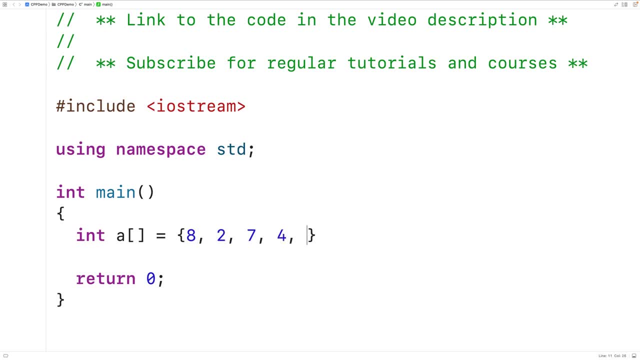 the unsorted values 8,, 2,, 7,, 4,, 5,, 1,, 9, and 3.. Now there's eight values in that array, so we'll declare and initialize an int variable called length to eight. We'll create a function. 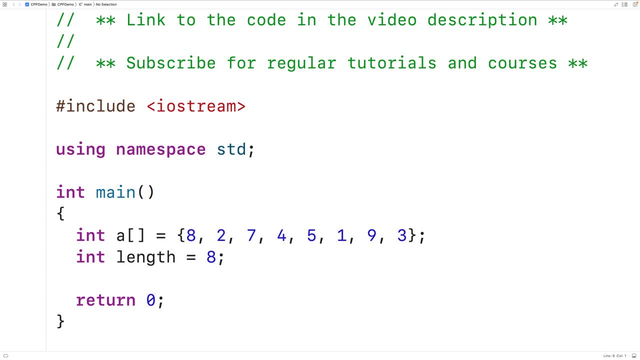 to perform the insertion sort algorithm. Here we'll declare the function. We'll call the function insertion sort. The function is going to have a void return type, because the function is not going to actually return anything. It's going to modify the array that it's passed as an argument. Here we'll have the array itself, Int a. 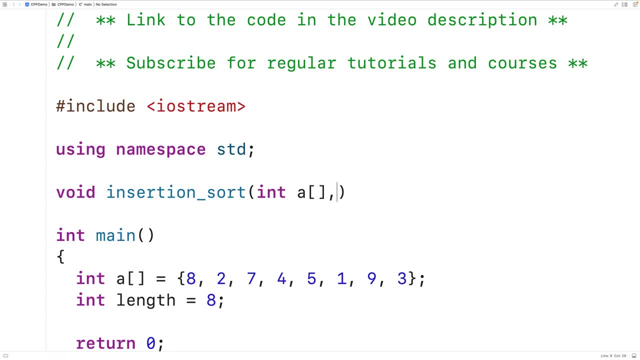 is what we'll call that parameter. The function will also accept the array length as an argument, so we'll have here int length for that parameter. We can then define the function down here. We'll copy this and insert it into the array. We'll call the function insertion sort. The function is going. 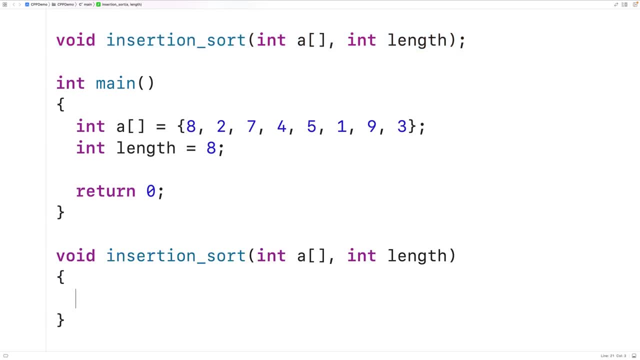 to paste this here and then we'll implement the algorithm by using a loop nested inside another loop. The outer loop is going to perform each major step of the algorithm by using a counter variable, i, to look at each key value from the unsorted portion of the array, The inner loop. 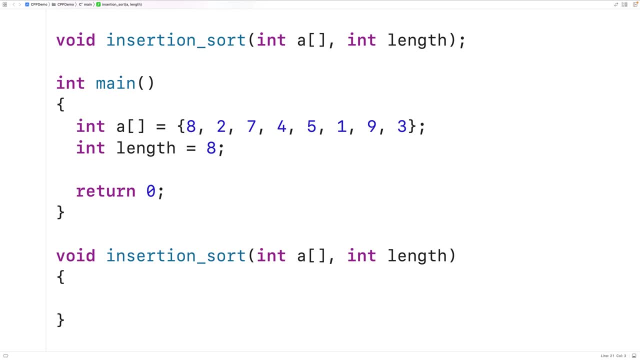 is going to use a counter variable j to help shift over the key value to its correct position in the sorted portion of the array. So first we'll create the outer loop with the counter variable i that's going to be initialized to one. It's going to go up until the length of the array and we'll 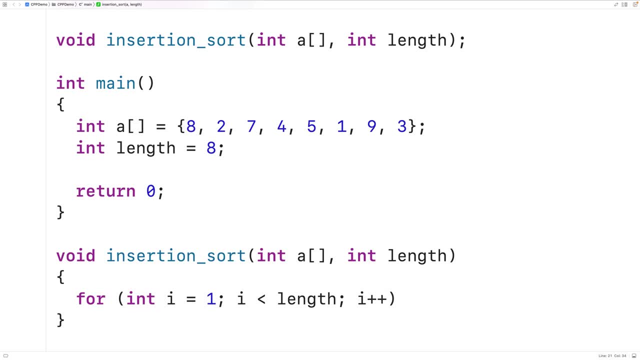 increment i by one. with each loop iteration We start i off at one, so that way the first key value we look at is the second element in the array. We're not going to look at this first element in the array. We're going to consider it to be already sorted because an array of one element 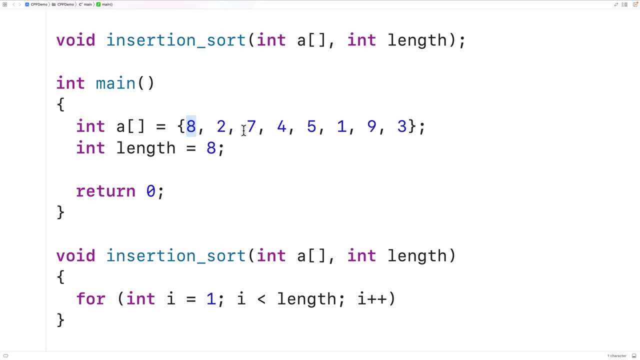 is sorted by default, Then i is going to be incremented with each loop iteration and we're going to do it like this. So i is going to be the last element in the array, Then i is going to be the next element in the right hand unsorted portion of the array until we reach the last element in. 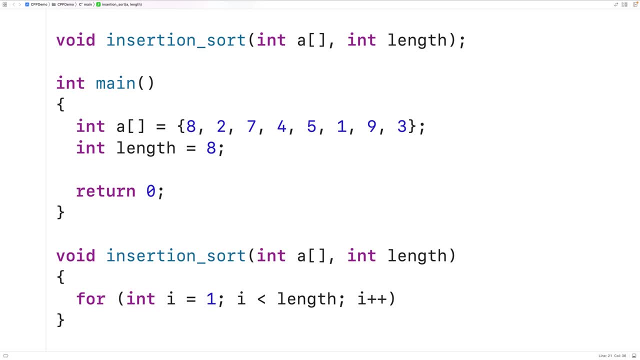 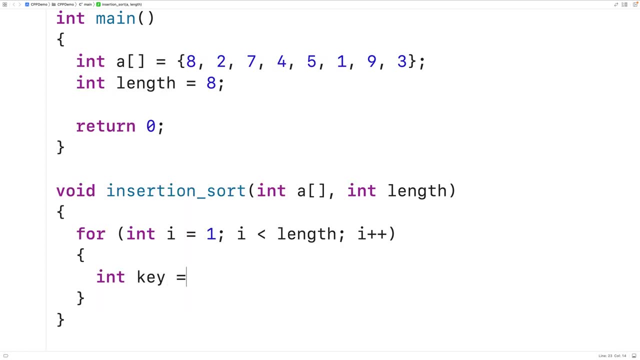 the array. So next we'll create the inner loop to shift that key value at the index i into its correct position in the sorted portion of the array. So here we'll have int- key is equal to a at the index i. Then we'll create a variable j to keep track of our current value. 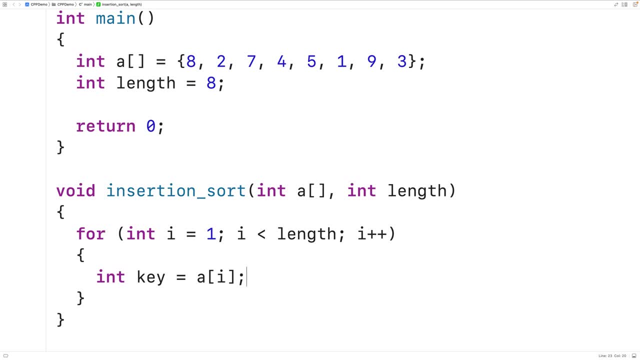 position in that sorted portion of the array as we shift over values. So we'll have here: int j is equal to i minus one, Because the value one index to the left of the current key value index i is going to be that first value in the sorted portion of the array that we're going to compare. 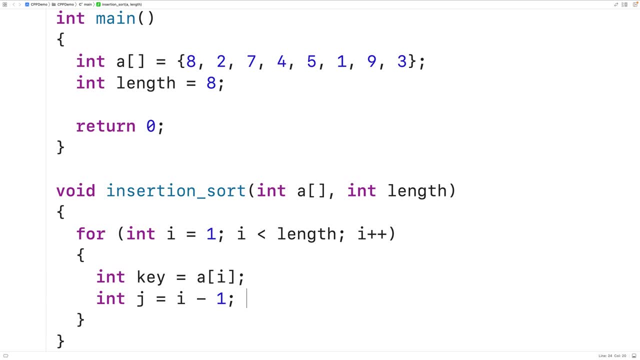 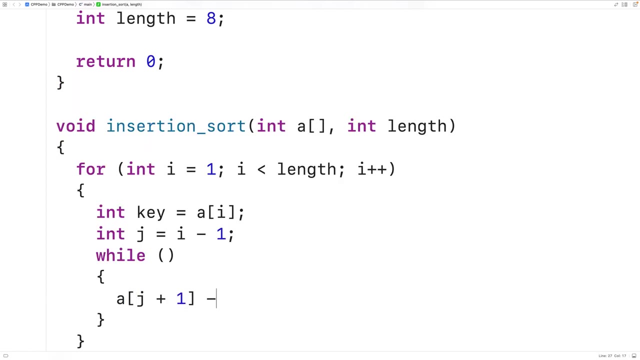 the key to. Next, we'll make a loop to shift over the values to the right by one in that sorted portion of the array. So we'll have here, while Then in the loop we'll have a at the index. j plus one is equal to a at the index j. Then we'll have j is equal to j minus one to update the. 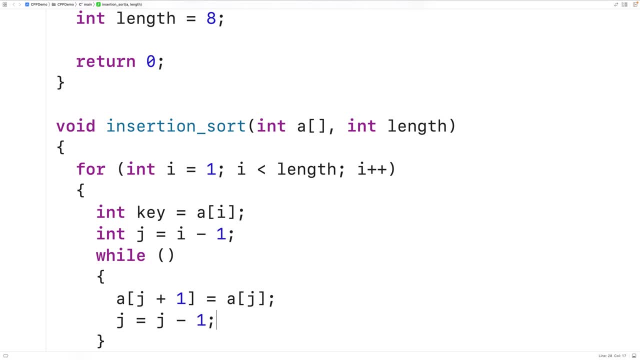 counter variable. So j is going to keep track of the index of the element that we're currently looking at in that left hand sorted portion of the array, And the index, j plus one, is going to be one in that left hand sorted portion of the array. So we'll have: j is equal to j minus one. 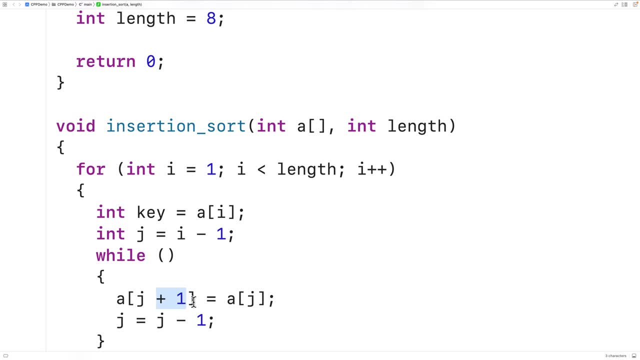 to the right of that current index j And we're assigning to that index the value stored at the index j, Which is going to have the effect of shifting that value over one to the right. Then we also decrement j by one with each loop iteration, So that way we keep on shifting over. 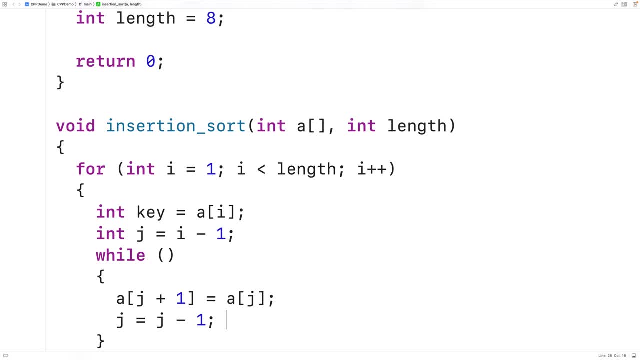 the next element in the left hand sorted portion of the array. Now we're going to stop this process if we reach the start of the array. So so long as j is greater than one Or equal to zero, We haven't yet reached the start of the array And we're going to keep this process. 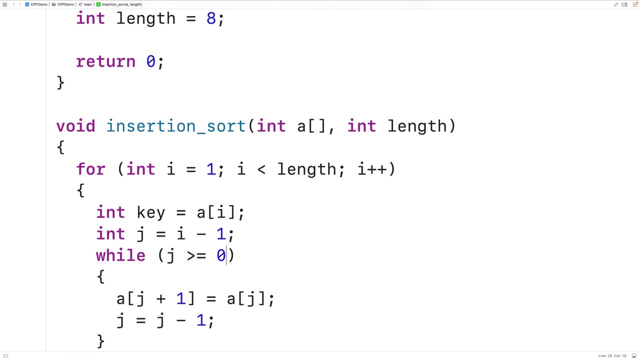 going. We're also going to stop if we find a value at the index j that is less than or equal to the key. So so long as we also have via and a at the index j is greater than the key, We're also going. 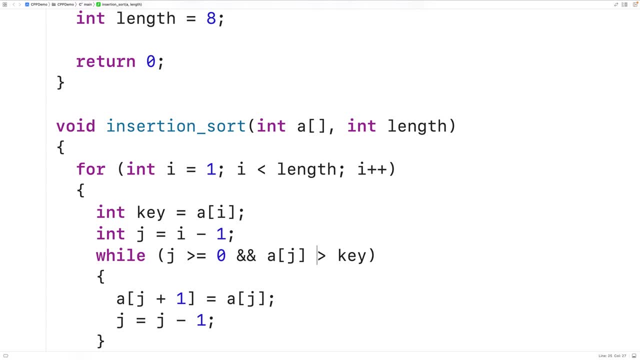 to keep going. So these conditions are going to determine when we found the right index to insert the key value at, Because if we reach the start of the array, That means the key value was smaller than all the elements in the sorted portion of the array. 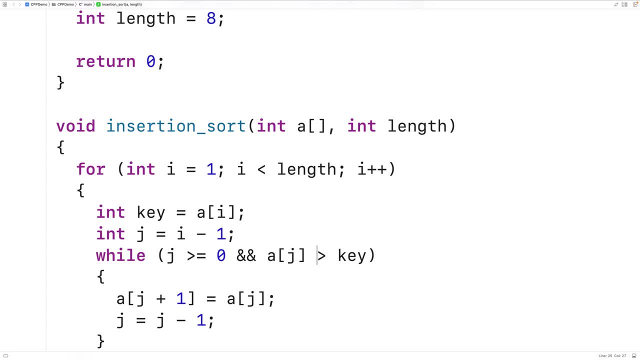 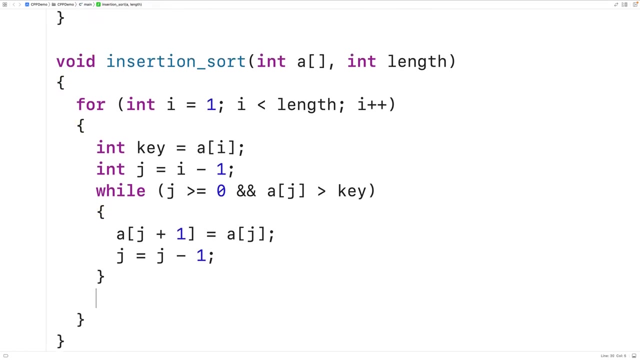 If the element at the index j is not greater than the key. We found an element that's either less than or equal to the key, And we know the key belongs at the index j plus one, One to the right of that element. And that's actually the next thing we'll do Is down here, After this loop, We'll have a at the index j plus one. 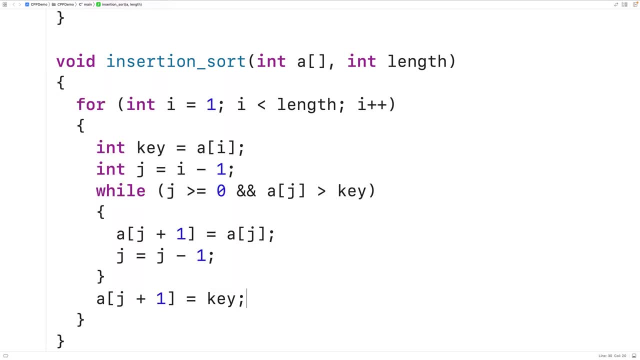 Is equal to that key value. Now, if we do reach the start of the array, It's going to be because j is no longer greater than or equal to zero. J is actually going to be equal to negative one. So here we're actually going to set a at the index zero equal to the key. in that case. 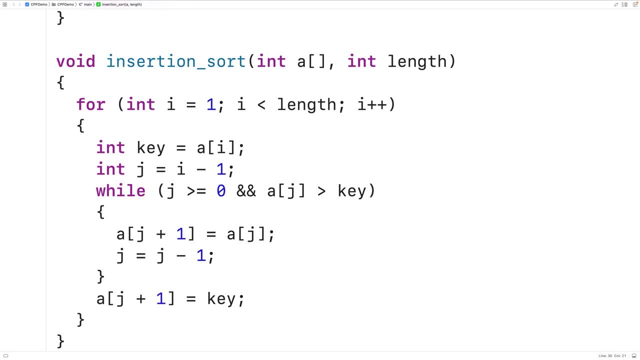 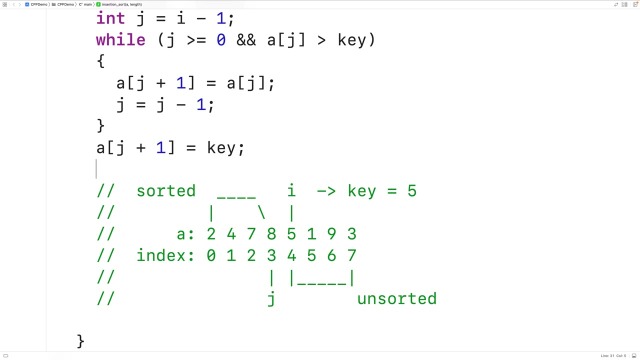 So this is actually it. The algorithm is now implemented. Let's actually step through one execution of this inner loop To help us understand what's really going on. So here I'll paste in some example. Here we have an array, And the array has the values two, four, seven, eight, five, one, nine, three. 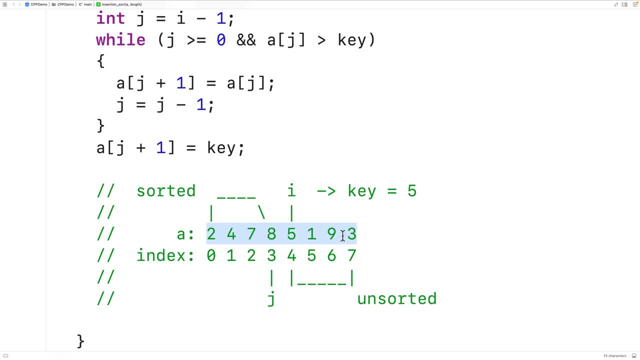 And the idea is that we're at this stage of the algorithm Where the index of i is four And so our key is five. And this here is the sorted portion of the array, And this here is the unsorted portion of the array. 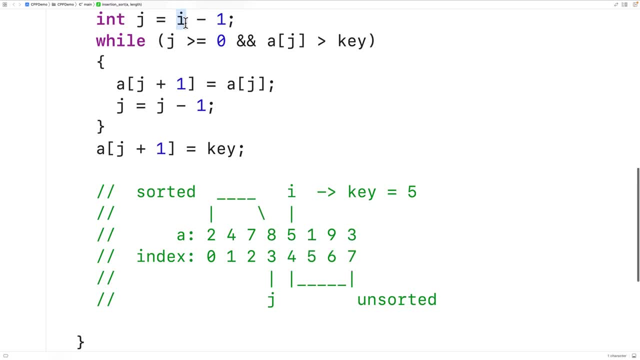 And because we set j to i minus one, That means here j is going to have the index three. So once this loop executes, J is going to be greater than or equal to zero, Because j is three, A at the index, j is eight. 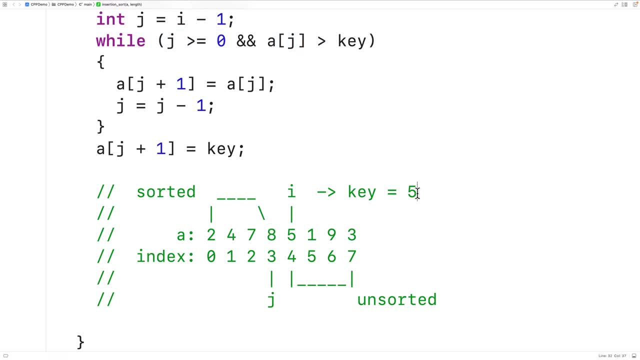 Which is greater than our key value five. So that means this loop body is going to execute And we're going to store into the index j, plus one Which is going to be four, The value stored at the index j. So we're going to take eight. 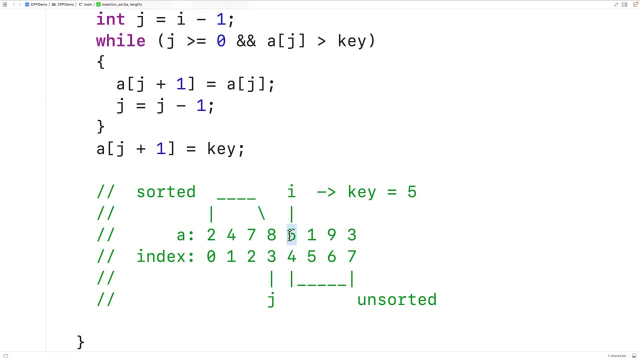 And we're going to copy it Here. Then in the next loop, iteration J is going to be decremented by one, So now j is going to be two. Then in the next loop, iteration J is still going to be greater than or equal to zero. 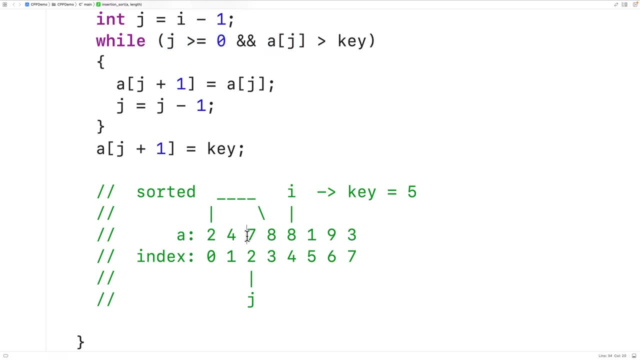 A at the index j is seven, And seven is still greater than our key value Five. So again, this loop body is going to execute And we're going to store at the index j plus one Which is now going to be three. 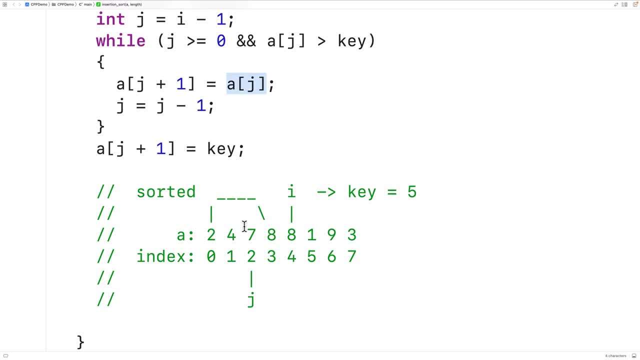 The value stored at the index j. So we're going to take seven And we're going to copy it here And again. j is going to be decremented Now, at this loop, iteration A at the index j is four, And four is not greater than our key five.